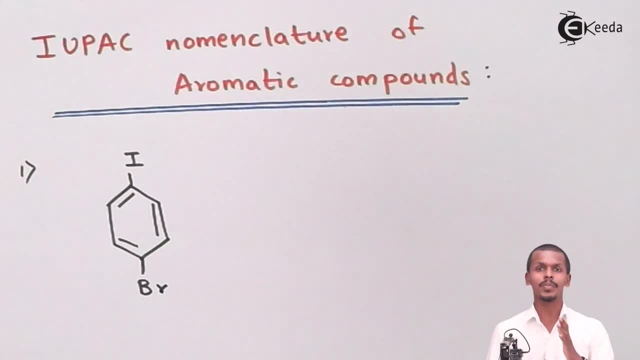 So in our case also, we have studied that the numbering should be done in such a manner that it should be in an alphabetical order. So in that case, suppose, in this case, in both the cases, suppose, if I take the number, that is, suppose, if I consider this as carbon number 1, this would be carbon number 2, 3 and 4.. 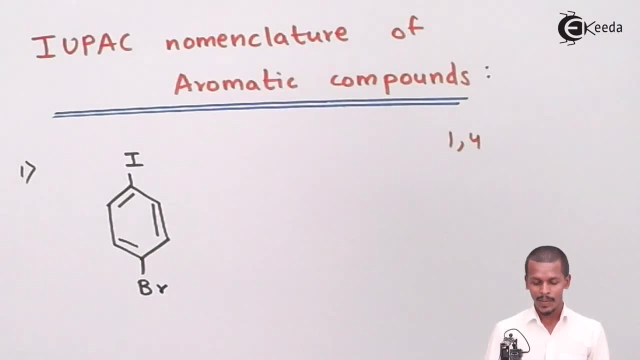 I would get a number as 1 comma 4.. But if I give it number from this side, that is 1,, 2, 3, 4, again I am getting 1 comma 4.. So from where should I consider the numbering Again? for this, the alphabetical order is the one that could help us out. 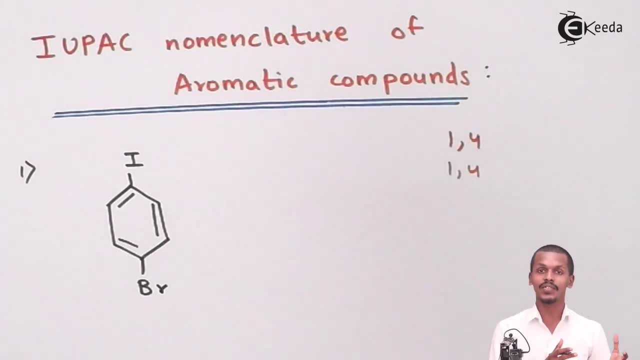 So therefore, the bromine is the one or the bromine atom. it starts with an alphabetical P, So that is the iodine it starts with. So therefore, according to the alphabetical order, we will give it the number to this one as 1.. So therefore, this one would be the second, third and fourth. 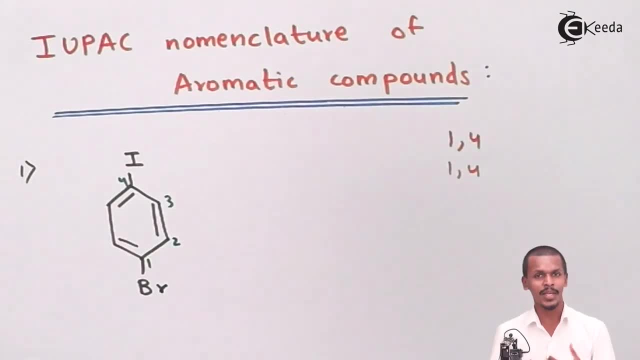 Even in this term also, we could analyze that- what would be the name of, or what would be the IEPC name of that particular compound. So therefore, according to this, the name of this would be: that is 1-bromo, and there it is 4-iodine and benzene. 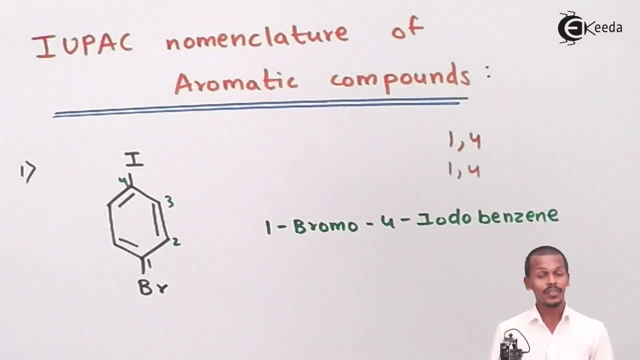 So therefore the name is 1-bromo-4-iodo-benzene. So now let us talk about the another one. So I hope this is the one that has been cleared and where we have given the correct numbering to the bromine atom and the iodine atom or the substituents. 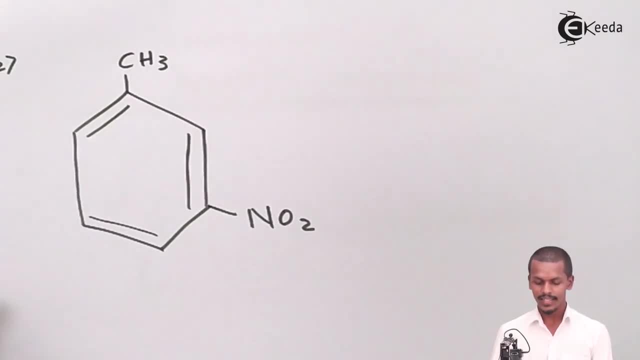 Now let us move on to the next one that we have. that is this one, And yes, it is again a disubstituted benzene And for which we have to give the numbering, But if you observe that I could give the number from that is NO2 also. 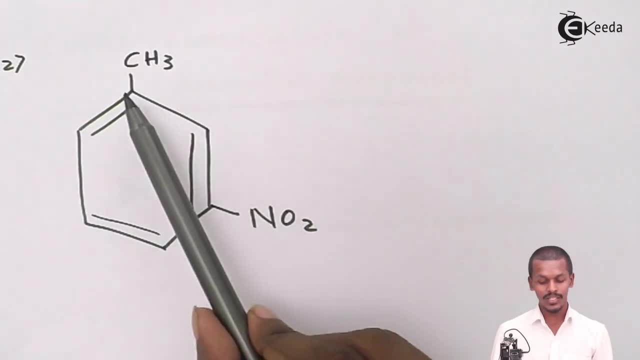 Suppose, if this is the carbon number 1, carbon number 2, this one would be carbon number 3.. And the number should not be in this manner where carbon number 1, carbon number 2, 3,, 4, 5.. 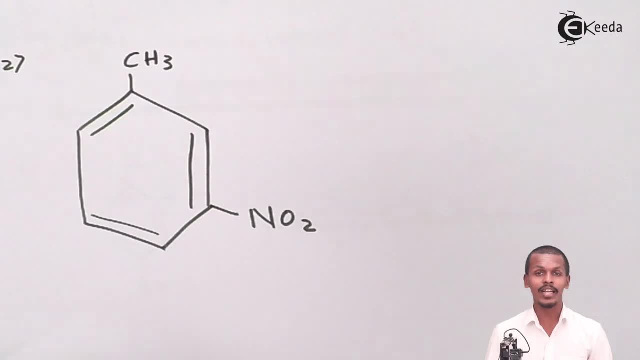 Then this term when we give it in anticlockwise. in this case, not in every case, But in this case, suppose if it numbers from the anticlockwise, then obviously we will get a bigger number, that is, 1,5.. And what if we have given the number from this one? 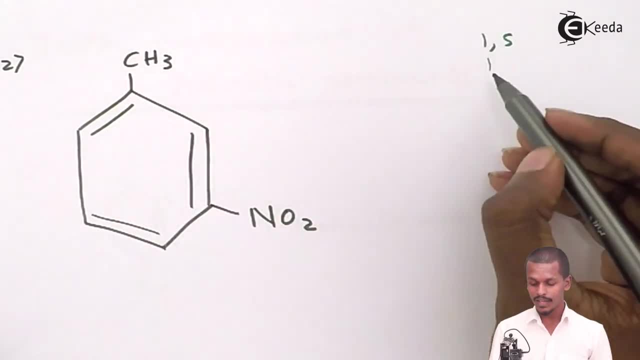 That is again and also in a clockwise suppose. if I will give it, then this one would be basically number it as 1,3. But if you observe that the special group is also been present over here, that is CH3 group, And we know that benzene and CH3 are basically known as toluene. 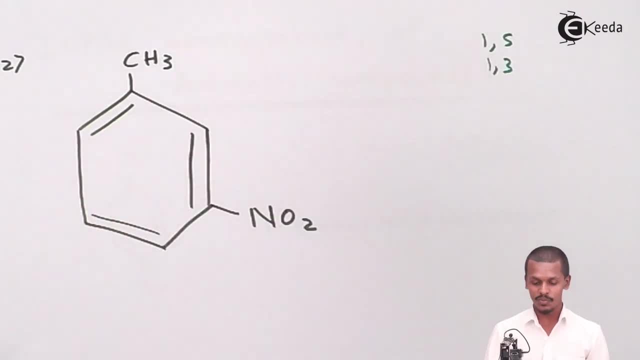 So therefore, since this is a special group, that has been a special compound that has been present over here, So therefore the number 1 will be given to the carbon atom Which has been attached to the methyl group over here. So therefore this is the carbon number 1.. 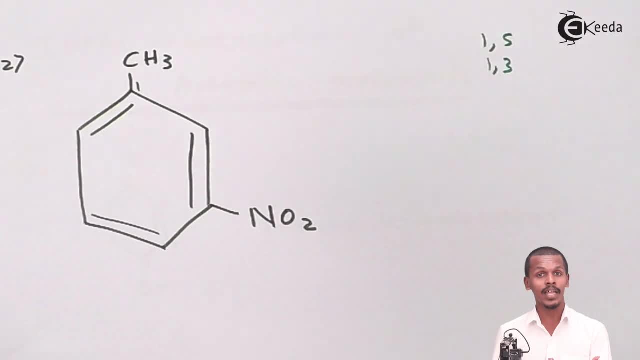 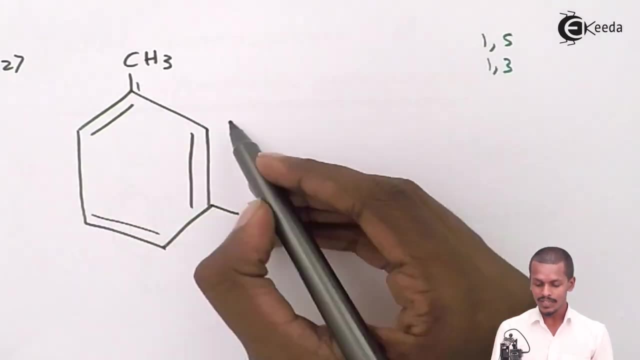 Again, I will do in such a manner and number in such a manner. where I could get the other number should also get a least number Or get less number of as it. okay. So therefore, this is the first carbon atom, This one would be the second and this one would be the third. 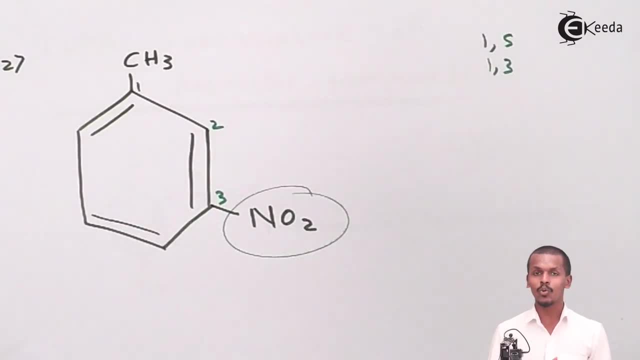 And on the third position, basically NO2 group has been attached over here And the special compound should end with its name, So therefore I could name it as, because this would be in the prefix form. So therefore the name of this would be nitro group. 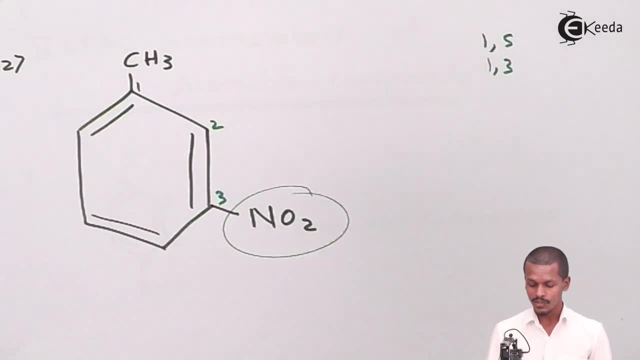 And that nitro group is present at carbon number 3.. So therefore, the name of this one would be 3-nitro, And the special compound is basically benzene plus CH3, which is known as toluene. So therefore the name of this is 3-nitro toluene. 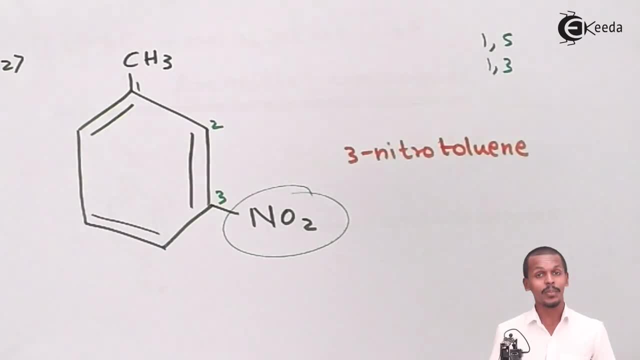 So this is the name, or this is the IEPC normalization that we have given to this compound. And now let us move on to the other one that we have. That is this one, That is this one. So again, we have got a disubstituted benzene. 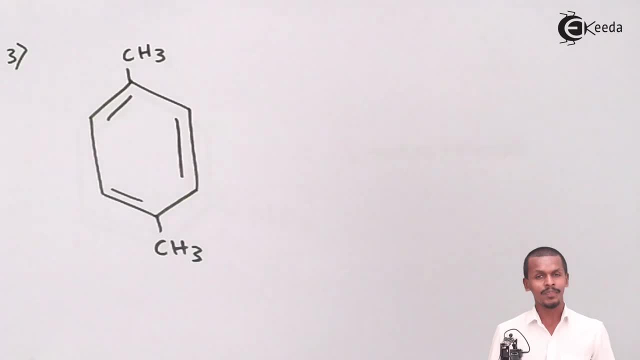 And in this case, as you could see that CH3 groups have been attached, But CH3 group, when it is attached to benzene, it is basically known as toluene, So therefore the special name should be given to this one. But we have also understood, that is, the rules of the disubstituted benzene, which we have got to know. 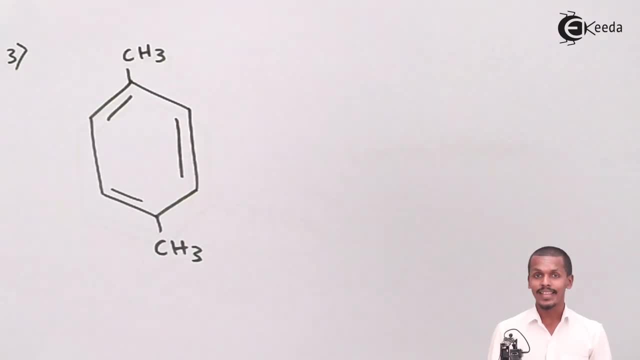 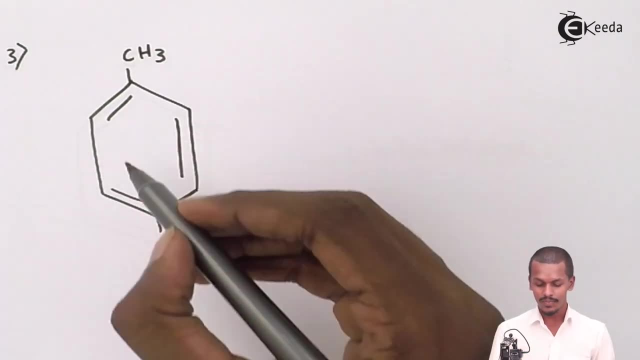 Suppose, if both the substituent group are the same, Then we should number it in such a manner that the ending should be end with this. So, for example, in this case I would give the number 1 to this carbon. Again, I could give the number 1 to this carbon also. 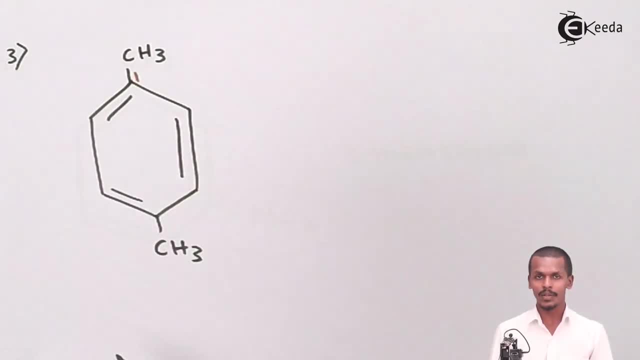 Because in any direction, if you give the number, then the combination that you could get is 1,4 itself, And the both are the same. So therefore, no case of priority that to whom I should give the carbon number 1 or carbon number 2.. 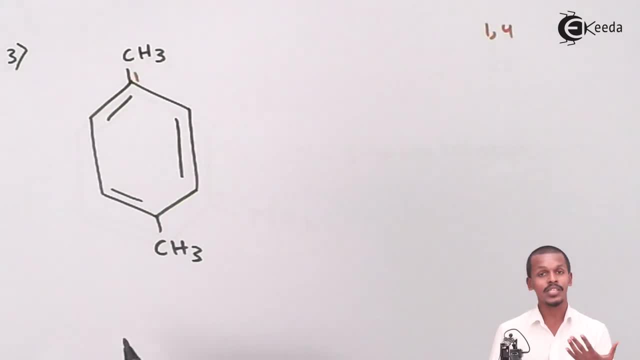 The substituents where it has been attached to. So, therefore, this is the carbon number 1 that we have, Again this is 2,3 and now this is 4.. So in this case, basically, the both the groups are being the same. 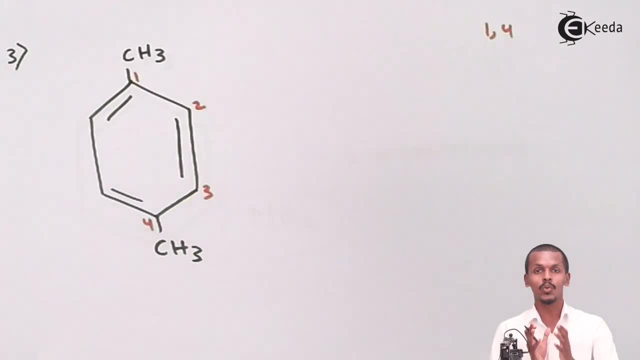 So that is the reason we should represent those groups earlier before the word benzene, And that is the reason that I could see that both the groups are present on carbon number 1 and carbon number 4. Making this to be called as 1,4 dimethyl. 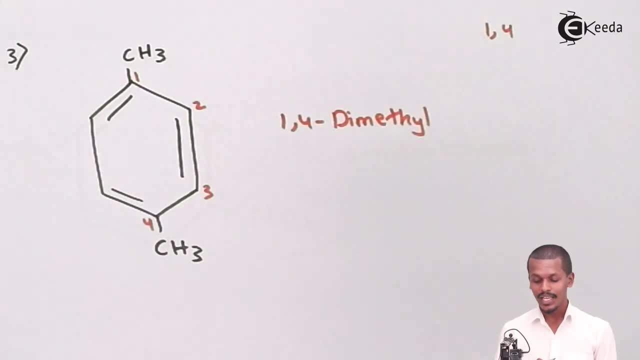 As, overall, it consists of benzene. So therefore, the name of this would be 1,4 dimethyl benzene. Simple one. Now let us move on to the next one that we have, That is this one. Now, it is not a bi-substituted or a dis-substituted. 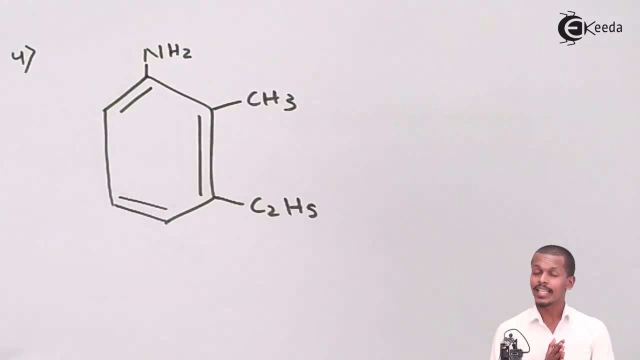 It is a tri-substituted, as we could see, And in this case the thing that we have to do is we have to number it, But the numbering should be in such a manner that the combination of the numbers that we have got should be very much less. 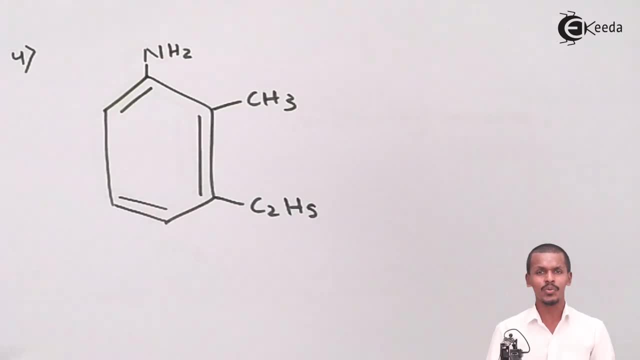 So, suppose, Because I am giving the different possibility that we could do and we could also be getting a wrong name. So for that suppose, if we have numbered it from this as 1. So I can't number this carbon as 2. Because it would give a long distance to this substituent and that will give a very larger number. 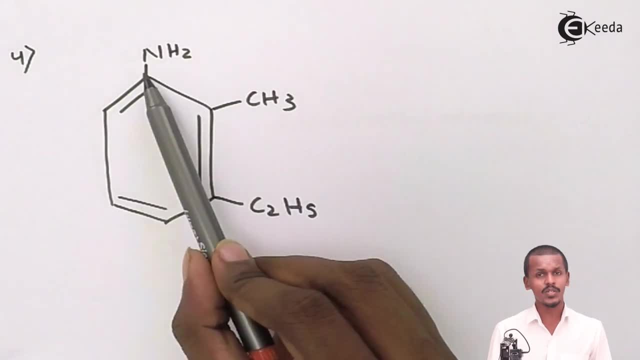 So therefore, the reason I have to give the number from this side only. So suppose if this is 1,2,3,4,5 and 6.. So the combination that I could get is 1,5,6.. So the combination that I could get is 1,5,6. 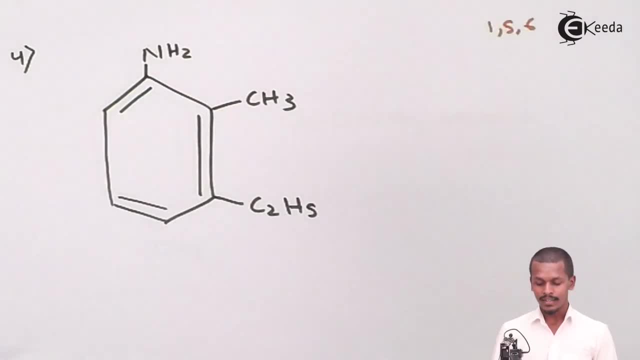 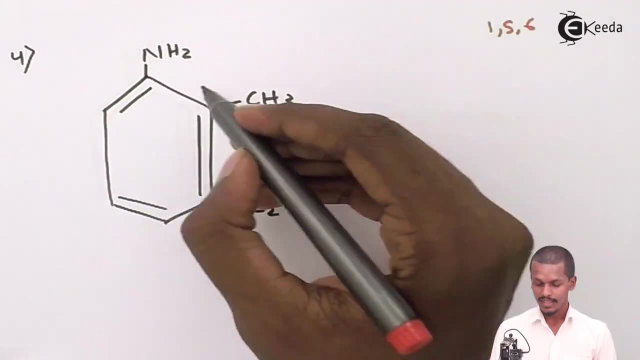 Which could be a larger number. And suppose what if I give the number from this direction, That is, from this direction, That is clockwise direction, Then this would be carbon number 1.. Carbon number 2.. Carbon number 3.. That is 1,2,3.. 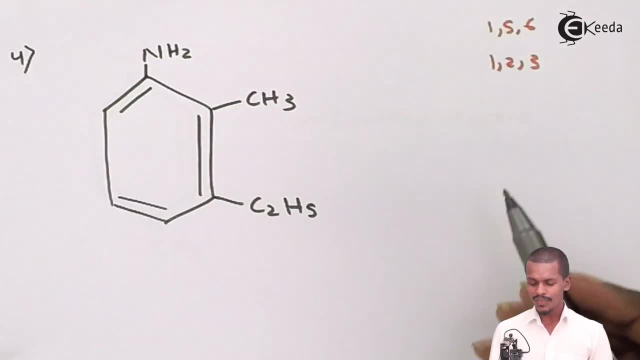 It seems to be a better option, But this is what we have got to know. that is, 1,2,3 is a better option, But the numbering will start from which substituent or which carbon atom which should be attached to the substituent. 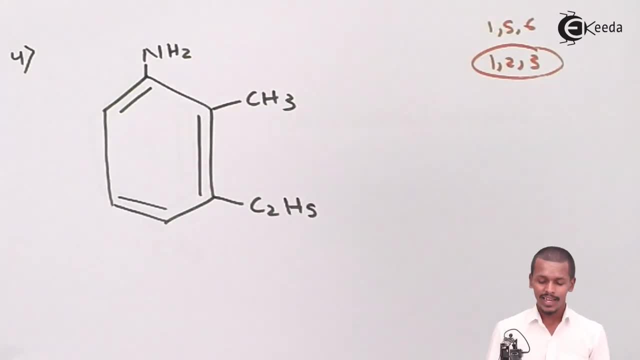 Is it C2H5 or is it CH3?? It is NH2.. Yes, because NH2, when attached to a benzene, it is basically known as an aniline, And that is the reason that the numbering will start. Even this was a rule of the IUPAC nomenclature. 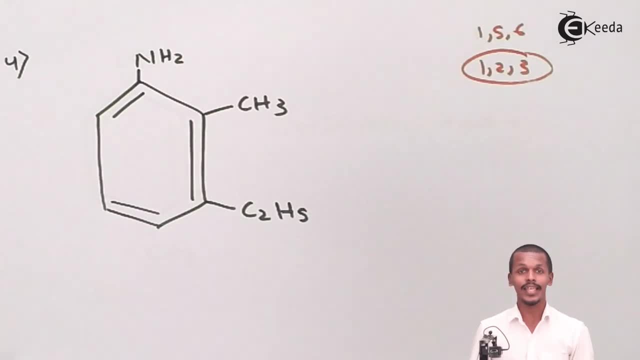 So this was also the rule of the IUPAC nomenclature that we have written for the aromatic compounds, And that is the reason that this makes us to get a special compound basically known as aniline. So therefore the numbering should be done from the group NH2 itself. 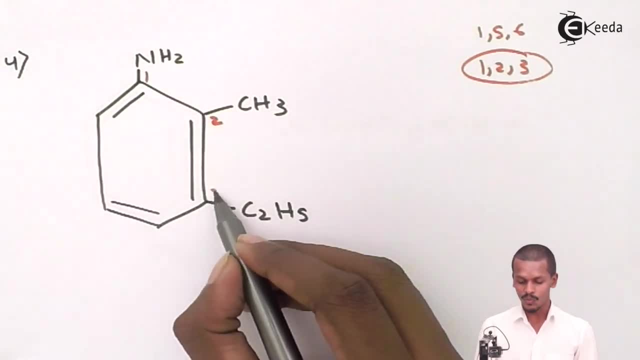 So, therefore, this one would be the group 1.. This one would be the second And this one would be the third. So, therefore, this is the numbering that we have written And talking about. what would be the name and what would we give the name to this compound? 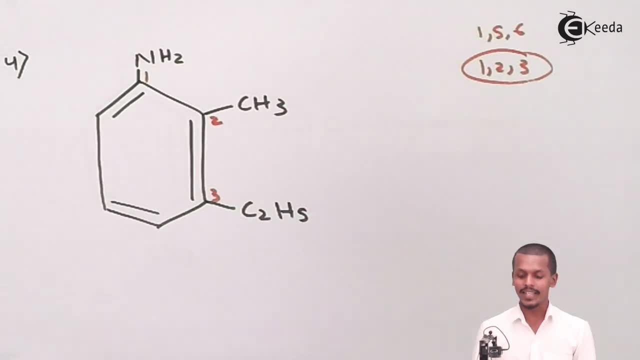 So in this case we could see that C2H5 is nothing but the ethyl group and on the second position it has been ethyl group. So we should write the ethyl group first. No, We could write, but the thing is we have to also obey the alphabetic law of order. 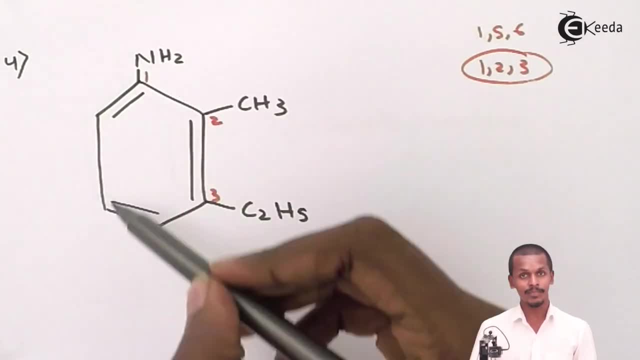 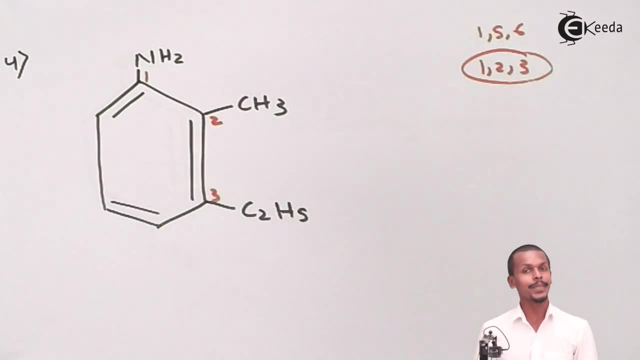 So, in that case, what we have got to know that these are the substituents, why this is the special compound that we have. So, therefore, we have only the two options that we have, that is, C2H5, and ethyl group, That is CH3.. 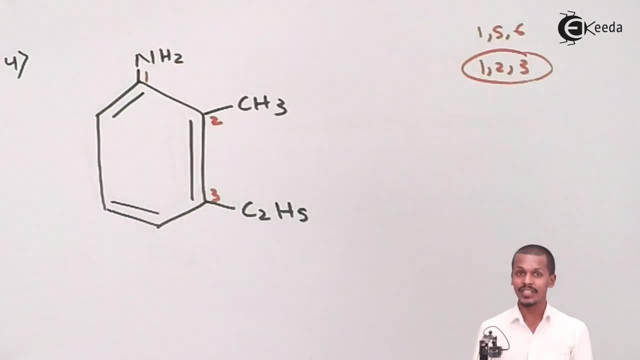 So the numbering has been done and the thing is we have to represent it and we have to insert a name to that, And that is the reason that of the third position is the ethyl group And the ethyl starts first compared to the end of the ethyl in alphabetic law of order. 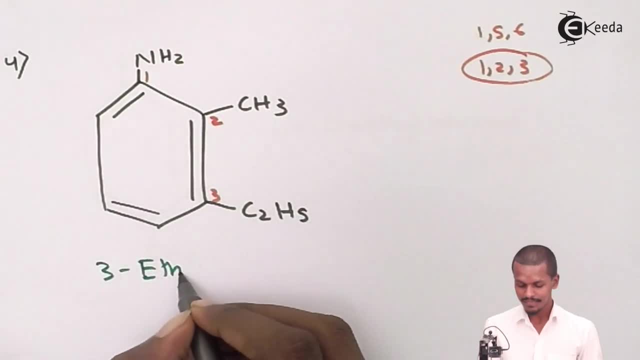 So therefore, we write it over here as 3-ethyl 2-ethyl, and the name of the aromatic compound is basically aniline, So that is why we have to write it as 3-ethyl 2-ethyl aniline. 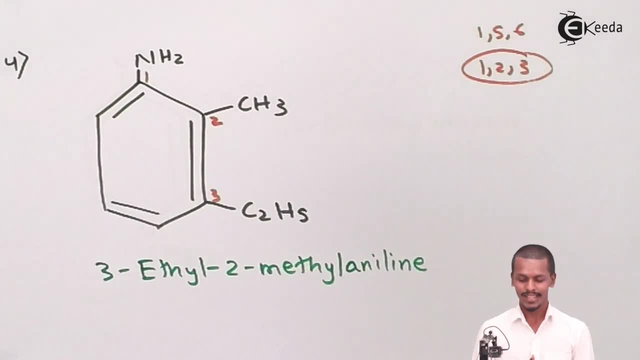 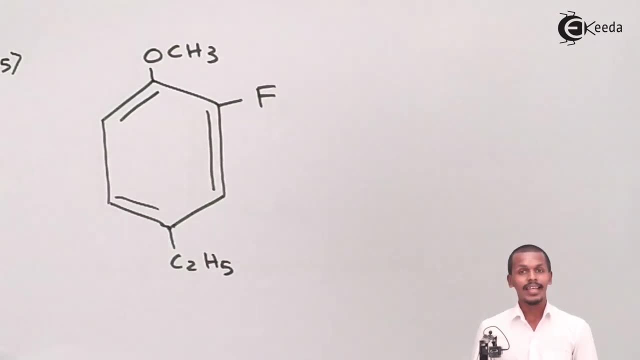 So this is the name that we have for this compound, and I hope you have understood this also. So let us move on to the another one that we have. that is this one, And this is the one that we have to give the number feature for this compound. 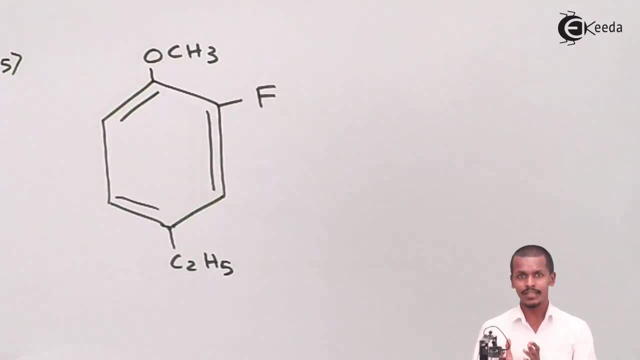 And yes, the thing is for the substituent. I think we have got to know that we should number from which direction and from which From which carbon substituent And in that case, suppose if we are talking about this one, then we should choose in such a manner that the less combination of the numbers that we would get 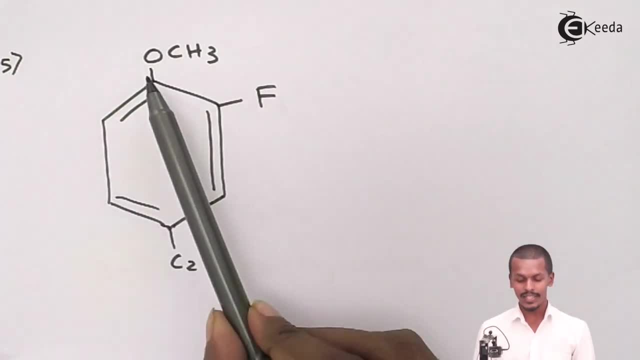 So I would get a less combination number if I choose either this one or either this one. So suppose, for example, suppose, if I am concerned about this number. So therefore this is the carbon number 1,, 2,, 3 and this one would be the 4.. 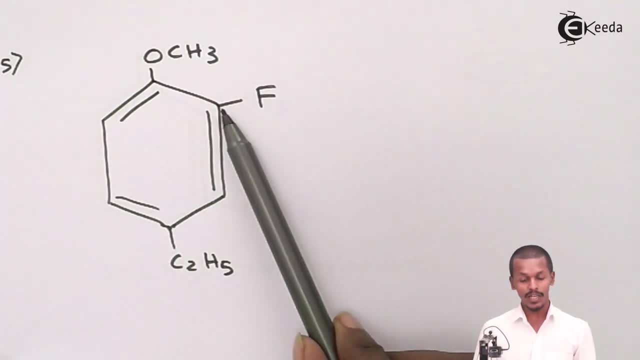 And what if I consider this as the carbon number 1.. So therefore, this is the one with carbon number 1.. So I would not choose this number. after that, I would choose this number. So because the combination should be less number that I could get. 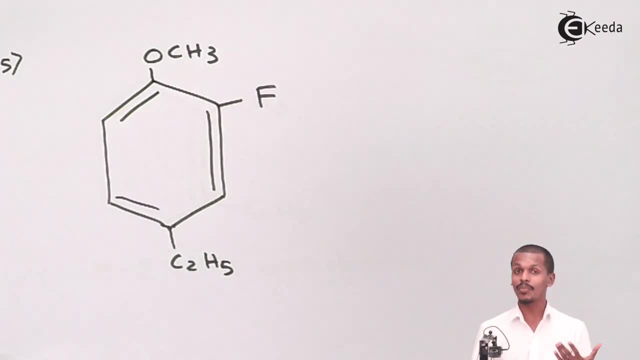 So therefore, this is carbon number: 1,, 2,, 3,, 4, 5.. So I am not getting carbon number, that is the 1, 2,, that is 4, but I am getting 1,, 2, 5.. 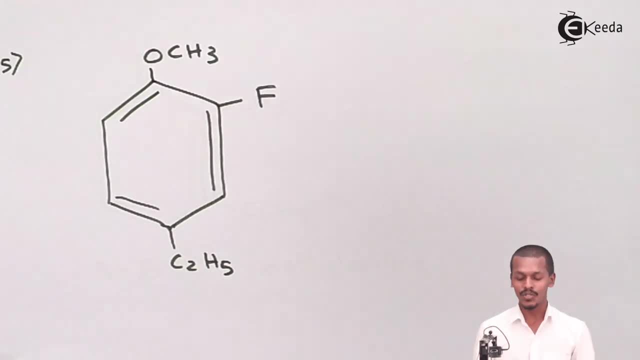 So obviously I cannot take even this one as the correct sequence of numbering. So obviously we have to choose a such a number where I could get a less combination of number And, moreover, we could see in this case that is the OCH3 has been attached. 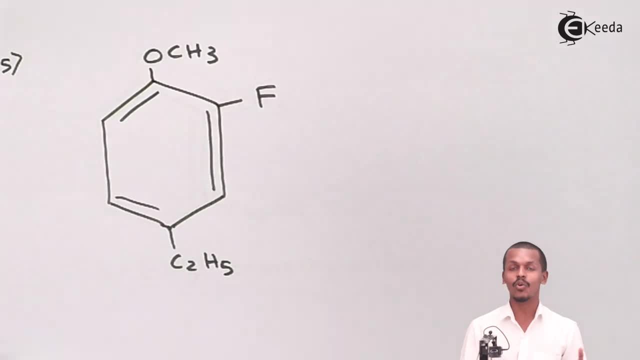 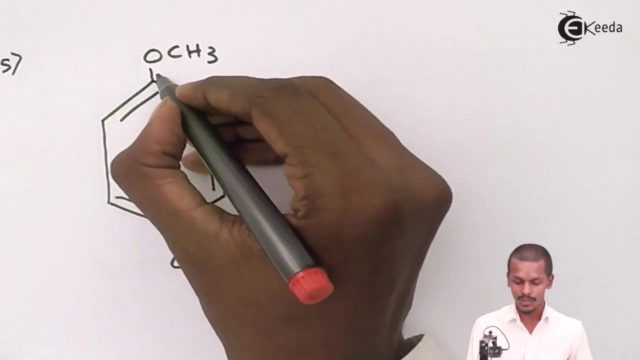 And this OCH3, if it has been attached to benzene, that is called to be anisone. Yes, that is also a special type of oil. that is also a common oil that has been approved by the IOBC nomenclature. So that is the reason that we will give the numbering from that special substituent, or, in this case, is this one OCH3.. 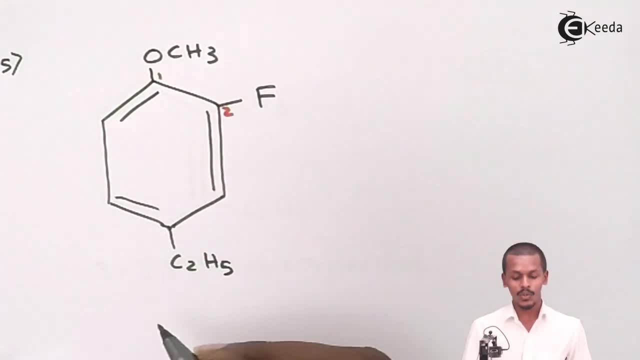 So, therefore, this one would be carbon number 1.. This one would be carbon number 2.. Carbon number 3.. And carbon number 4.. So this is what we have And talking about, because this is the substituent or basically the anisone is the one that is basically the special compound that we could get. 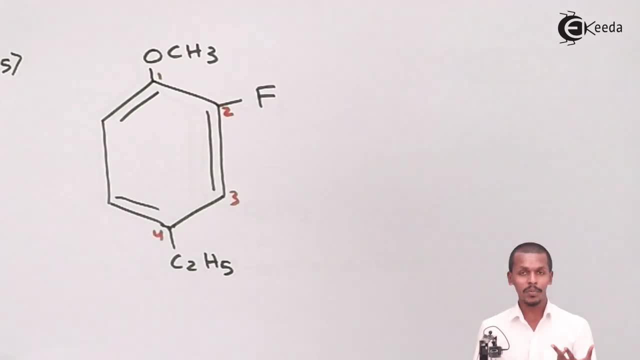 And that is really the reason that we have only two options with us, so as to have a combination that which one we should write first and which one we should write later on. And that is the thing that ethyl is the one that it starts with E. 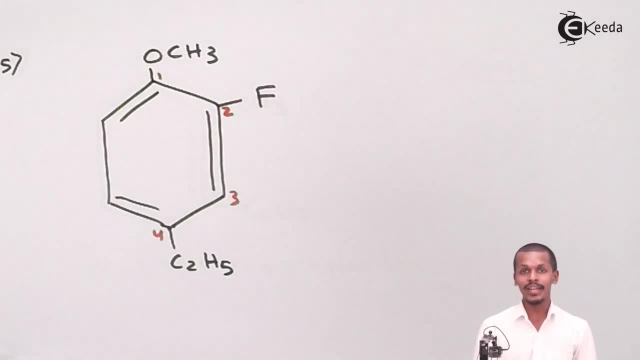 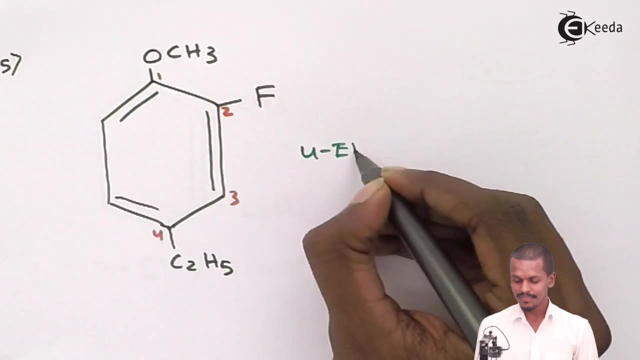 While fluorine is the one that starts with F. Making an alphabetic order give you a preference to ethyl first, So that is the reason that we could write the name of this structure as Four ethyl, And on second it is chloro group. it is predestined. 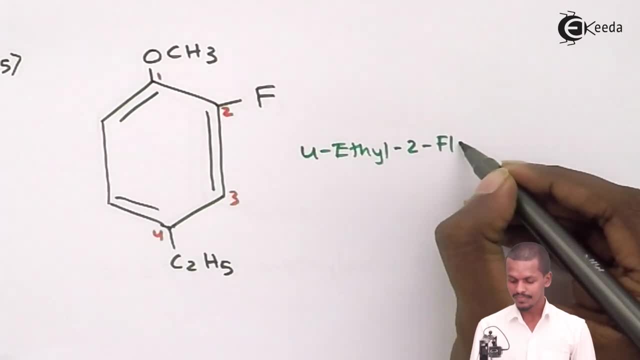 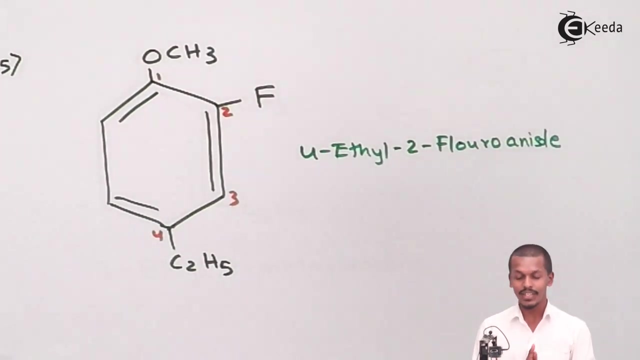 So therefore four ethyl, two fluorine, And the next is basically because it is an anisone, so therefore we could write it as Anisone. So therefore the name is we clearly mentioned over here, that is the four ethyl, two fluorine anisone. 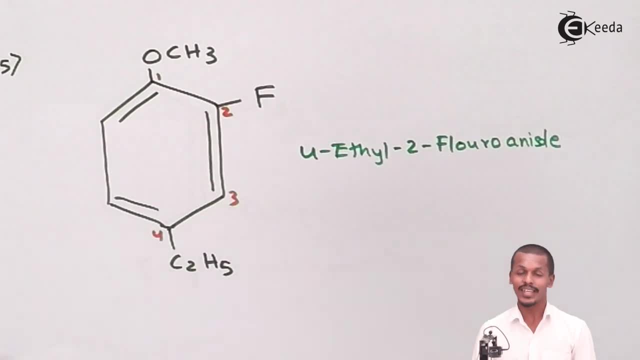 So that is the name of this compound that we have, And let us talk about the next one, This one, And let me give the preference that I hope you have got to know that, from which we should give the number at. This is basically a tri-substituted benzene. 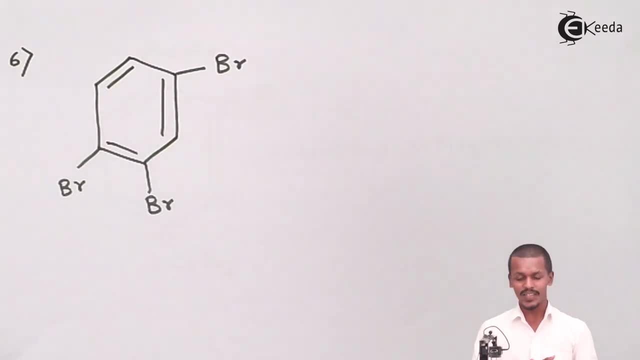 We could say that all these, all the benzene substituents are basically are the same in this case. Basically, this is the bromine atom, And even all these are bromine atoms. So the number it should start from which at, Because that is the main thing. 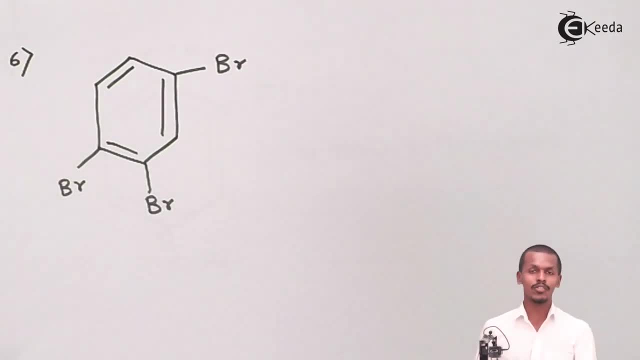 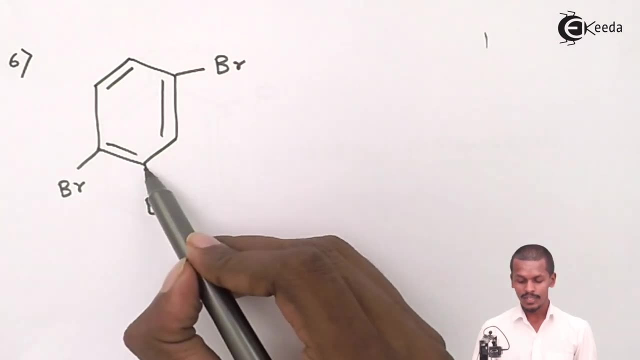 So I should choose in such a manner that the less combination of the numbers there I could get. So suppose if I choose this number as carbon number one, Then this would be carbon number one: Two, Three, Four, That is one comma three comma four. 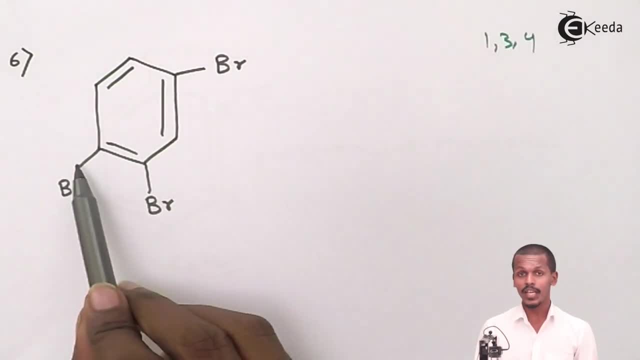 And what if I choose the number from this? So therefore, this one would be carbon number one, Carbon number two, Three and four. So among these two, One comma two comma four is the best option. So that is the reason I will number it in this form. 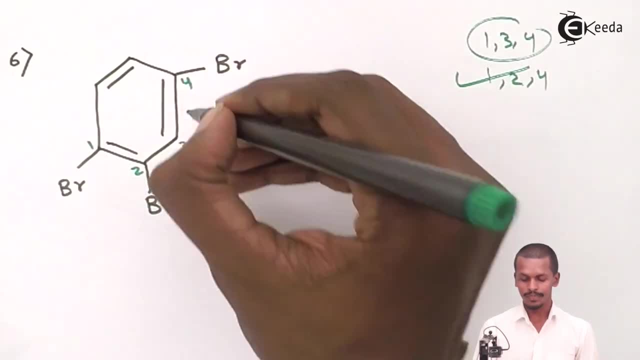 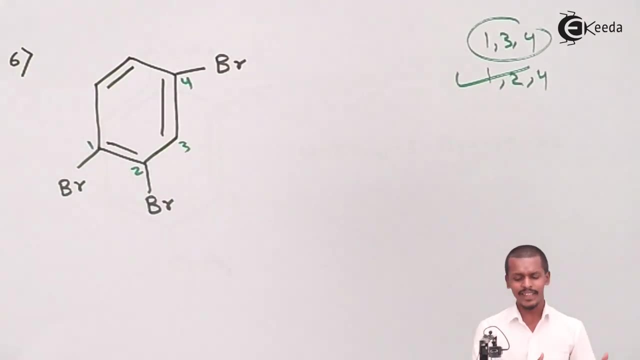 This is carbon number one, Two, Three And four, And since all the substituents are the same, So that is the reason we have to represent all the substituents first, And then we will give a better name to this aromatic compound. 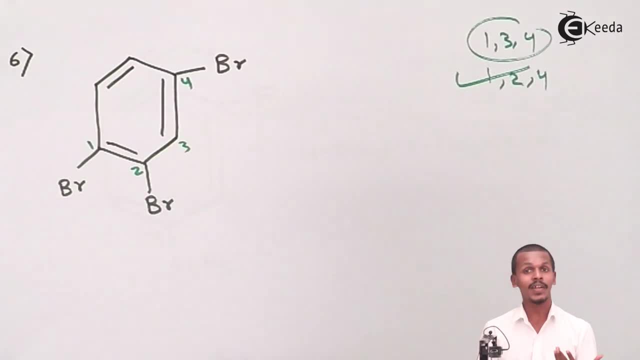 So therefore all the groups that are the same over here is basically bromine That are being attached on the first, Second And fourth of the carbon atom of the aromatic index of the benzene. So therefore I could name it as one comma, two comma, four.